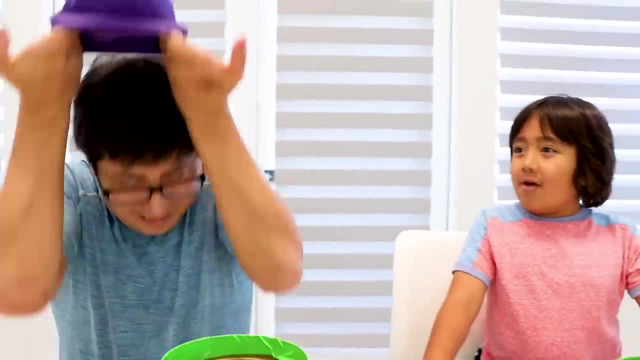 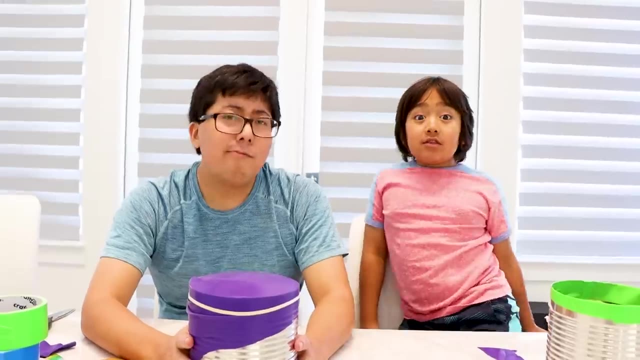 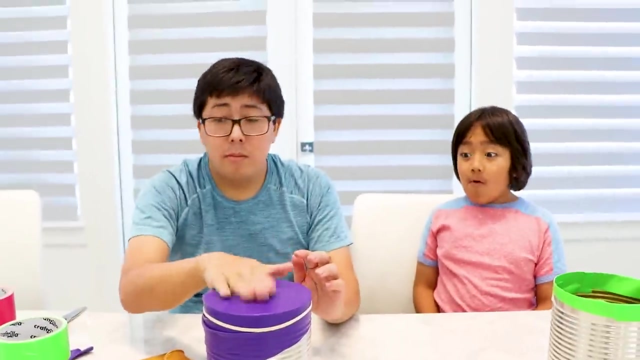 This looks like a swimming head cap, right, Yeah, Put it over here. You can also use rubber bands to hold the balloon in place. Now it looks like a drum, And now for the other drum. Alright, this is a special one, It's golden. 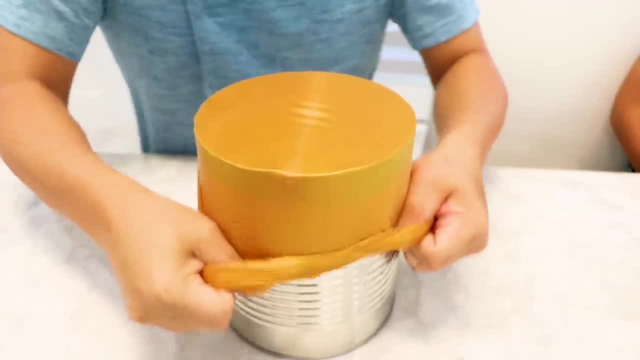 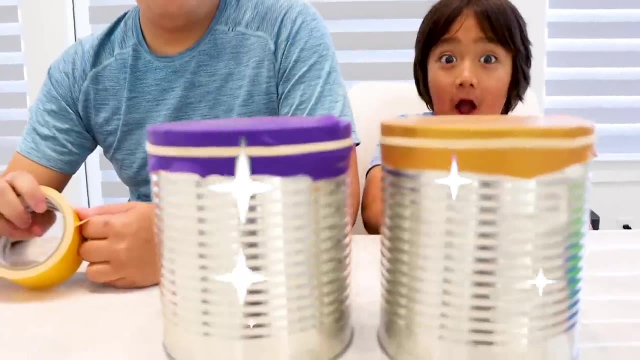 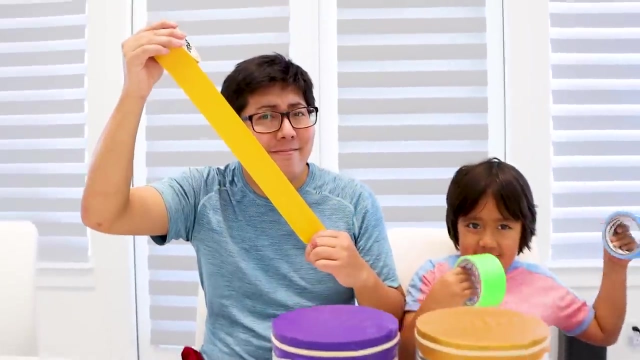 Alright, It's done. Now we're going to cut off the extra balloon pieces. Next we're going to put tape around the keys to do decoration. Alright, We have to go all around. Ryan, can you just give me a minute? 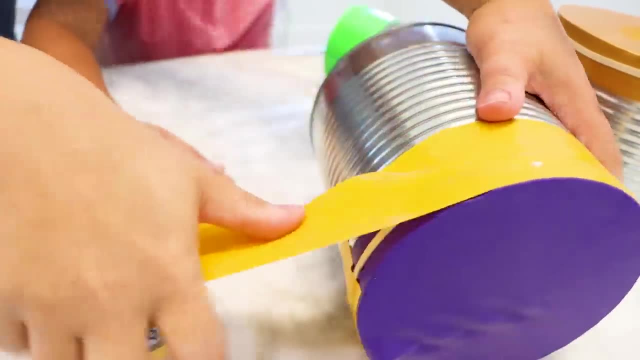 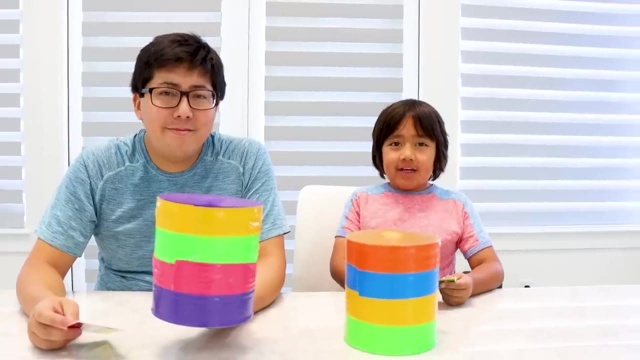 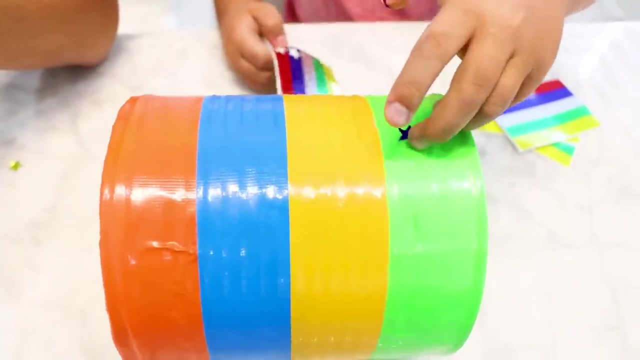 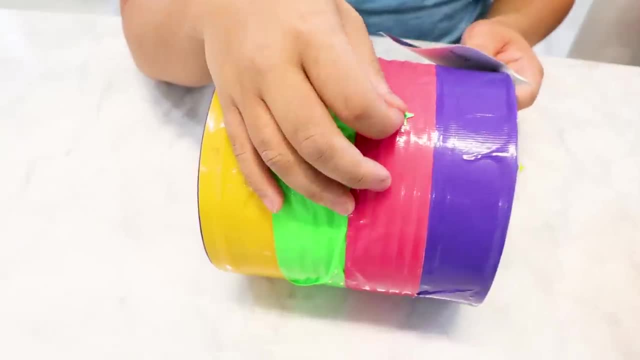 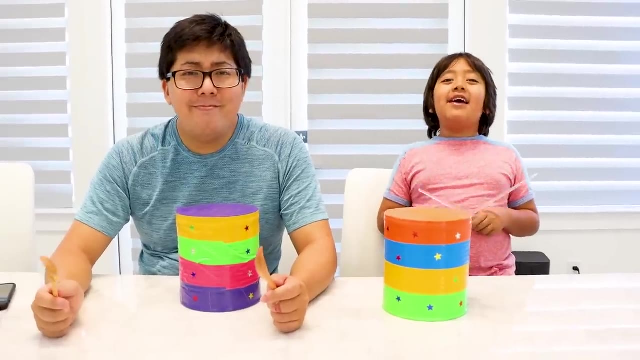 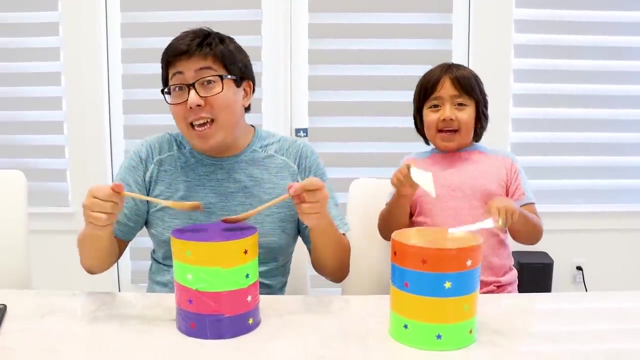 Put it right here: Green, star and yellow. Okay, guys, it's done, Let's jam. I hate the music. I'm going to build a robot. It's going to be my best friend. I'm going to build a robot. 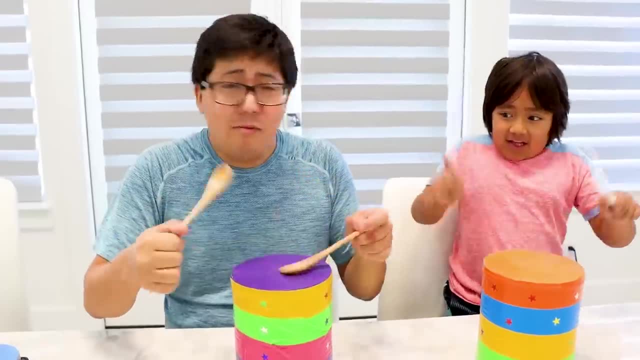 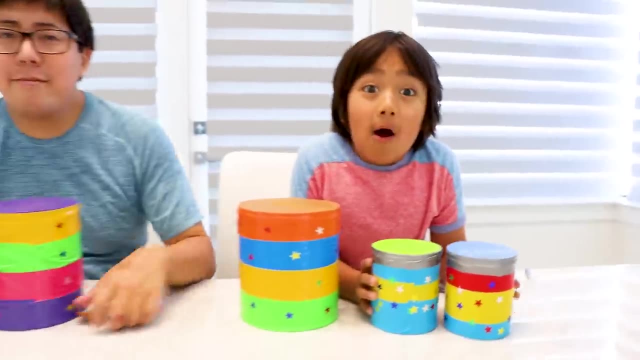 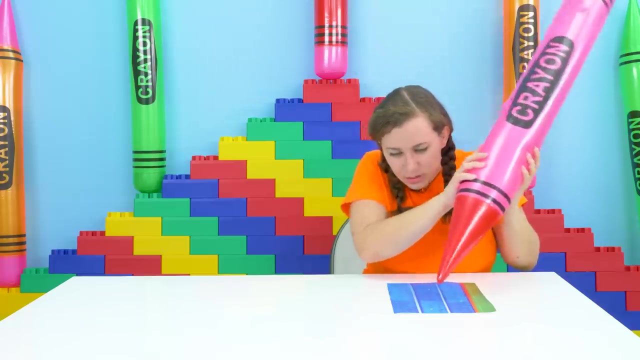 Grab some tools and let's begin. You can also make a smaller version like this: Come on, let's go And let's show Peck. Alright, let's go. Whoa, Oh, Whoa, Hey Peck. 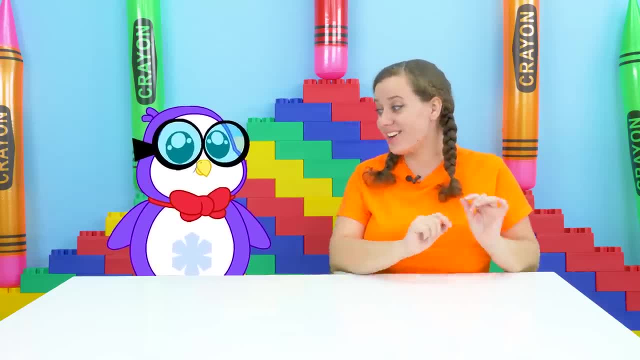 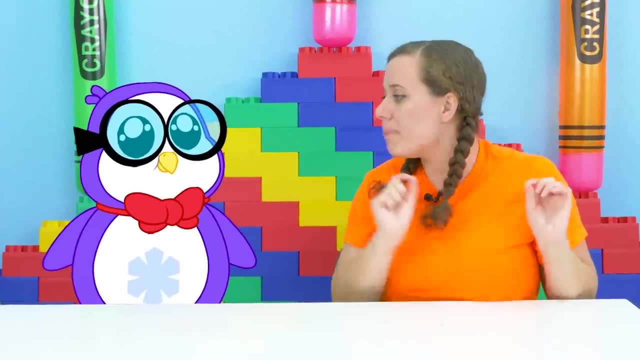 Wait a second. If you're here, does that mean that Ryan sent us a new project? That's right. We got to make some musical instruments. Musical instruments, Oh man, that sounds like so much fun. I bet we could find things around the house to make them with. 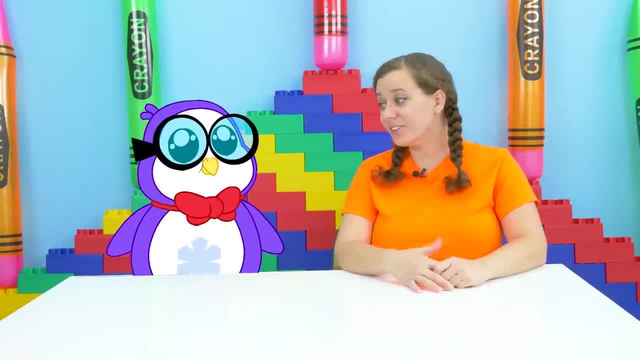 Let's find some things to rattle, make noise and do other fun stuff. Yeah, no, that sounds great Peck, But we should probably get going Like an instrument that uses strings. But we can go find these things. 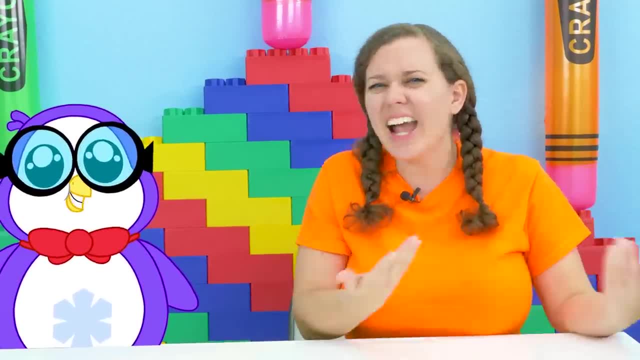 How about one that you have to blow into, which will make it a wind instrument? I think I'm just going to go. I'm just going to go. Okay, Oh gosh, Where did Peck go? I got to go get supplies too. 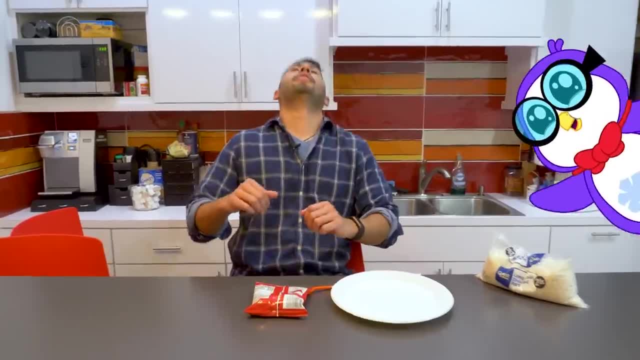 Whoa, Whoa Man. what a hard day of work. It's time for my snack And it's Cheez-Its. Here we go, Cheez-Its all over my plate. Now teeth this with my trusty spoon. 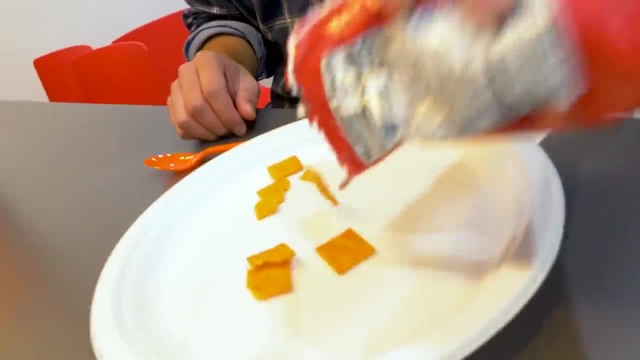 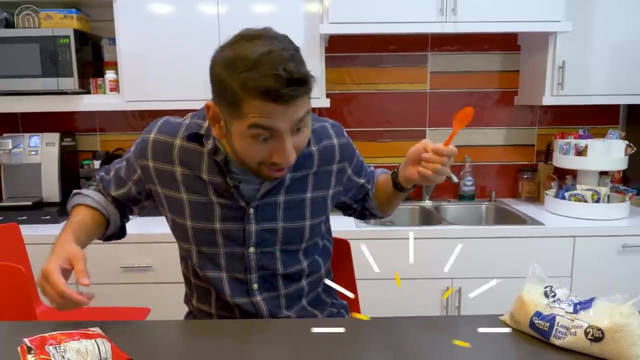 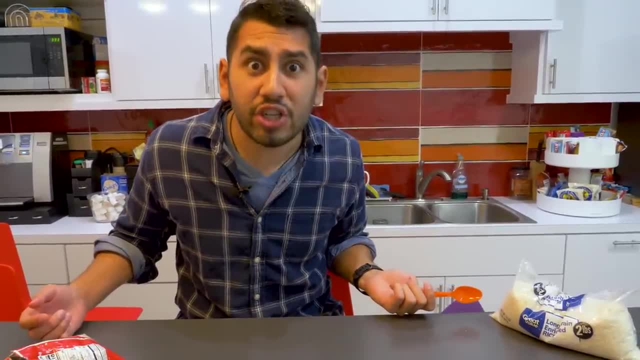 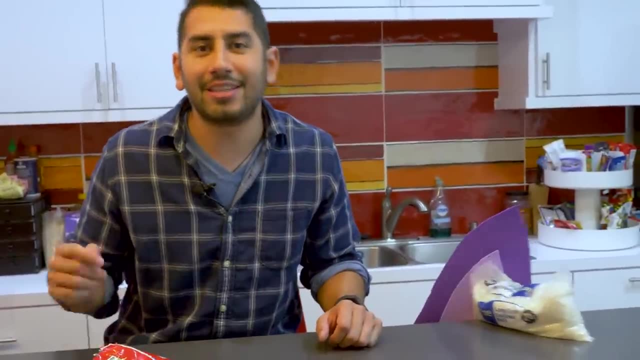 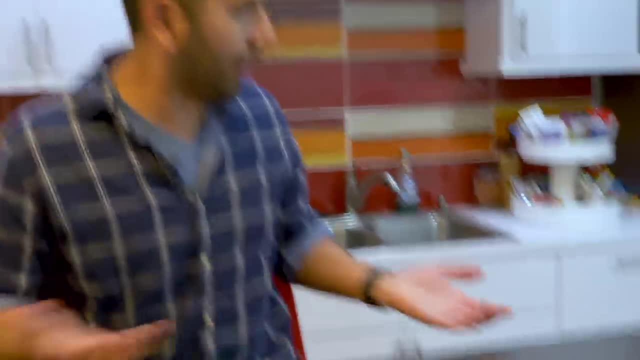 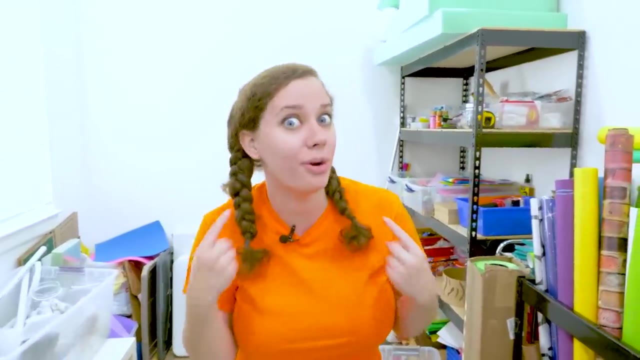 At least I still have my long grain and wrist rice. Wait, Where did my rice go? So, while Peck is doing whatever it is that he's doing, I know the perfect place to start. Come on, come on, come on. 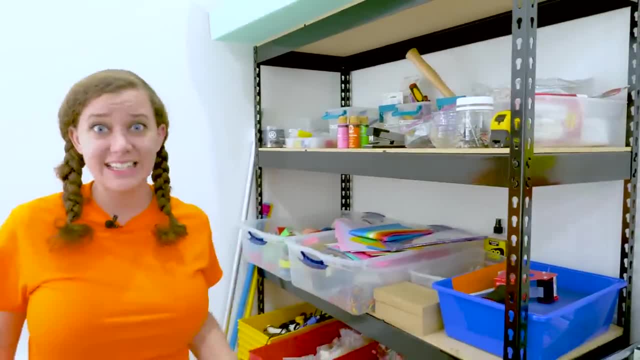 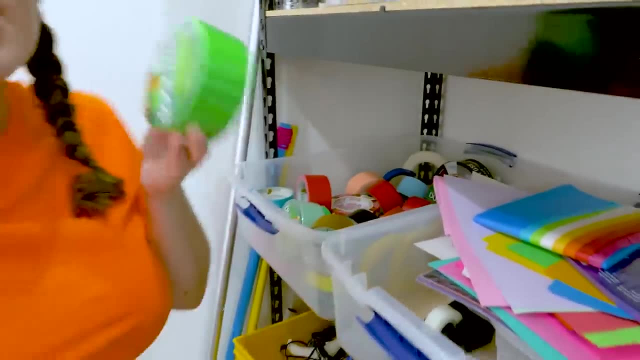 Okay, we have this whole shelf full of all sorts of arts and crafts and things like that. There has to be some good stuff in here, So let's see. Oh, first of all, We need tape, and this is so bright and fun. 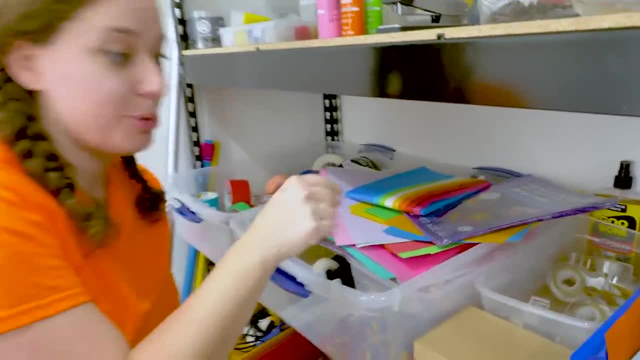 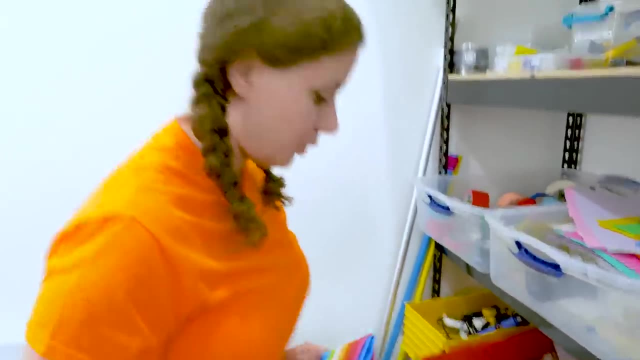 Okay, maybe we could use some rubber bands. I mean, you can do anything with rubber bands. Let's get all of those. Definitely some colorful paper. I think that's a great idea. And, ooh, I wonder what's in here. 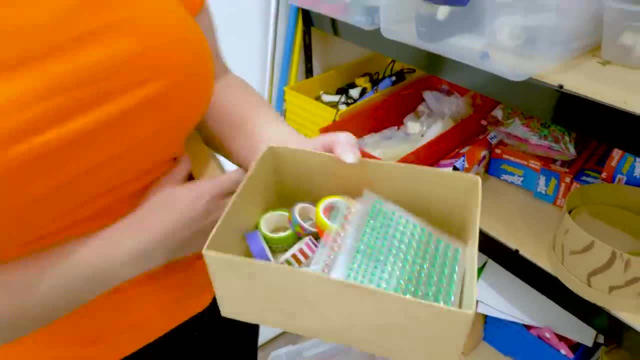 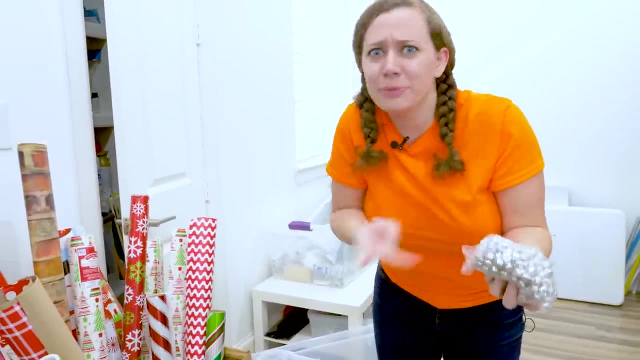 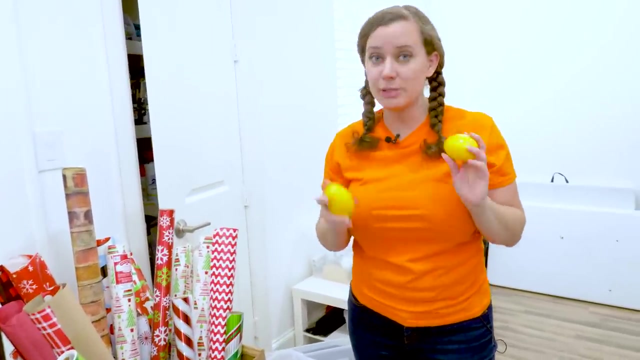 Oh look how pretty and sparkly everything is. I don't know what we're gonna use this for, but we're definitely taking this with us. Jingle bells- That's pretty much an instrument already. Eggs- I don't think somebody put this back in the right spot. 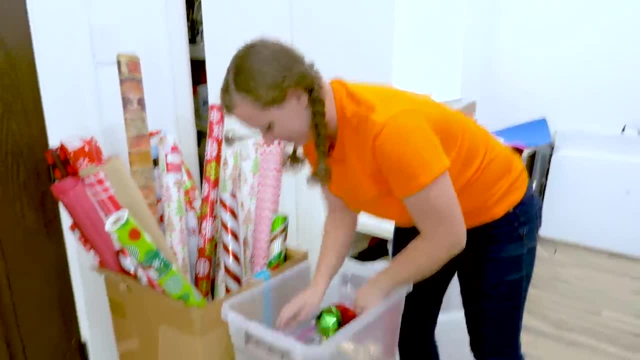 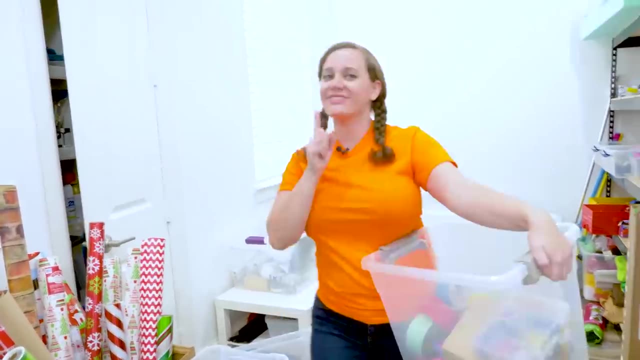 but I think we could use these too. What else do we have? Wait? a second Thumbtacks. Well, they're bright and colorful. I think we can use those too. The last thing we need I know what. 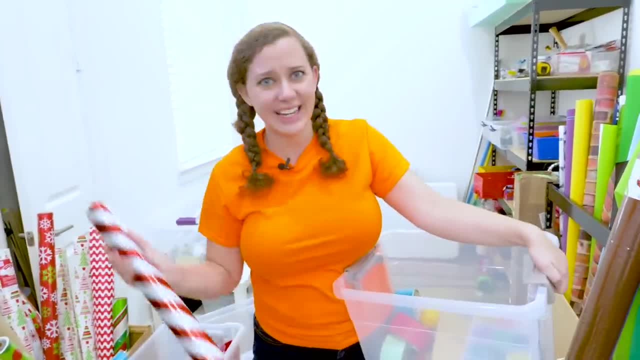 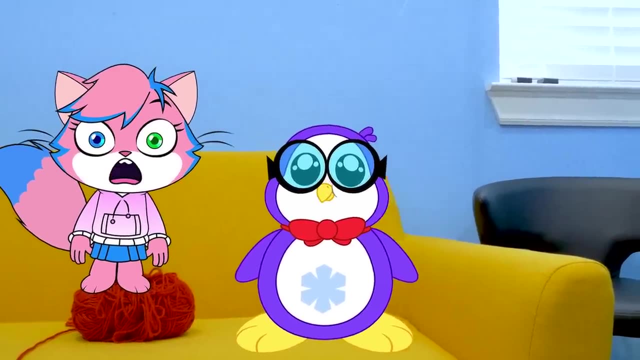 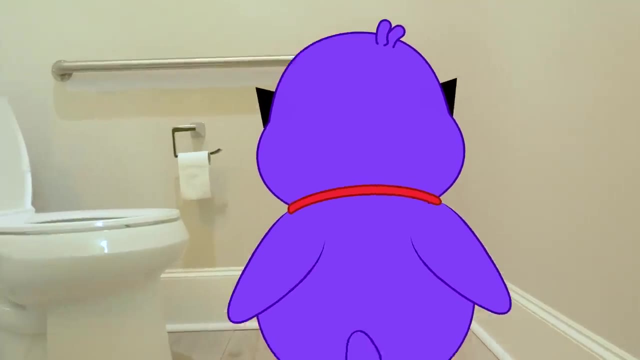 Wrapping paper. This is perfect. I have everything I need. I wonder what Peck is doing. Ooh, what do we have here? Yarn, I can use that. That, Yeah, Aw, That's so silly. Yoo-hoo-hoo, woo. 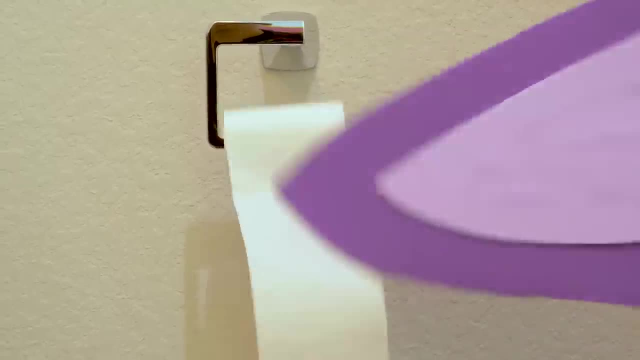 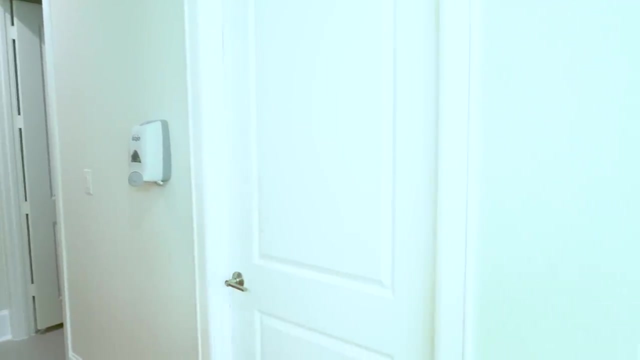 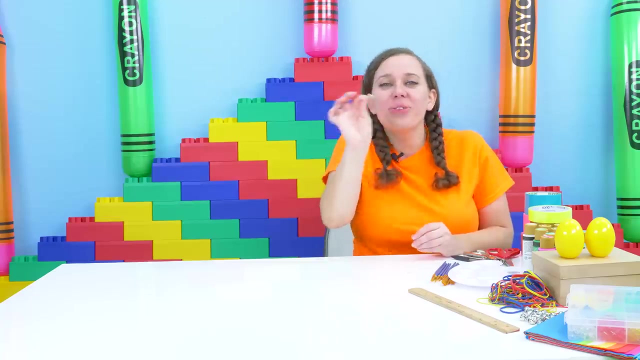 Just gonna borrow this toilet paper roll, And there we go. Yeah, Oh hey, Peck, Wait, Where's all the toilet paper? Sorry, Daniel Peck, It's the world's tiniest toilet Peck. 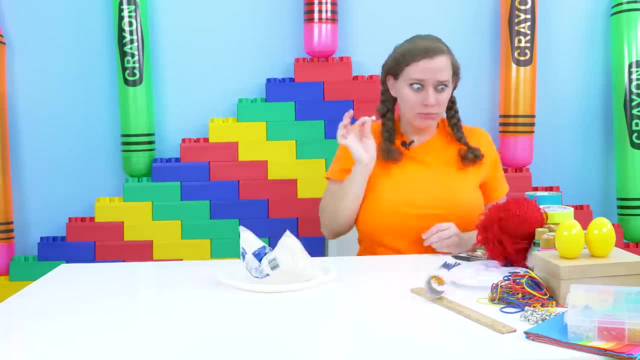 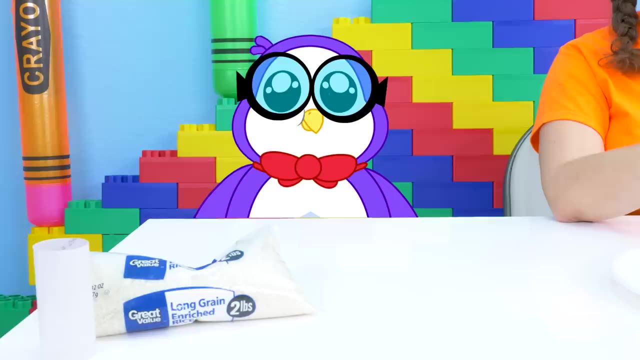 It's the world's tiniest instrument. Aw, Incoming Peck, I found some things that we can use for instruments. Yippee, The toilet paper roll. What if you started with a tambourine, One of my favorite percussion instruments? 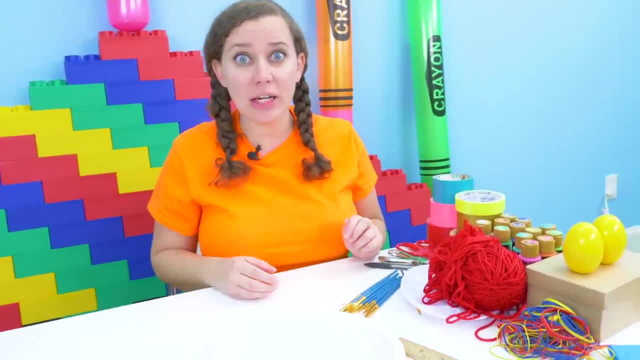 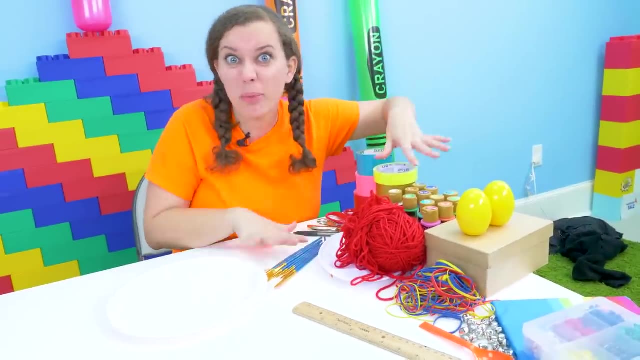 That's a great idea, Peck, And it looks like we have everything we need. For starters, we can use this plate to be the base, But it's kind of white and plain, so we can paint it- maybe some bright, pretty colors. 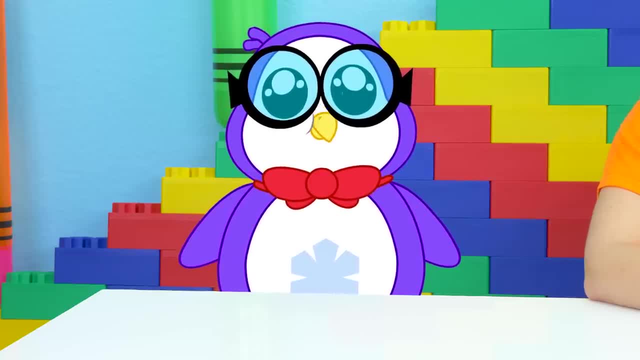 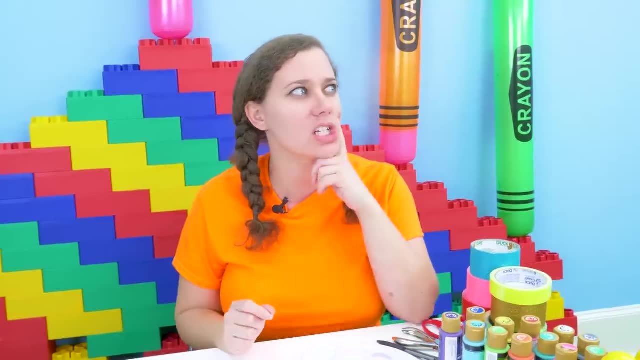 I don't know how that's going to work, but I believe in you, Bree. Oh, I have the perfect idea. What is more colorful than a rainbow? So we need all the colors of the rainbow, which is ROYGBIV. 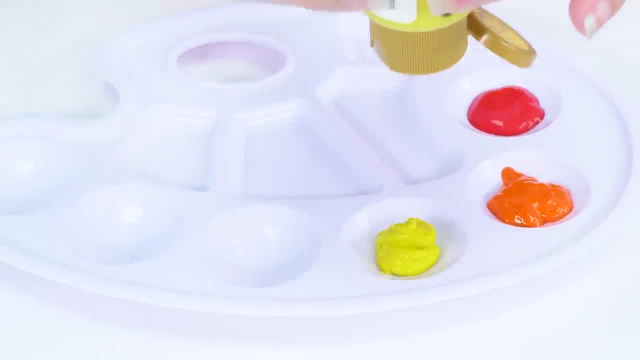 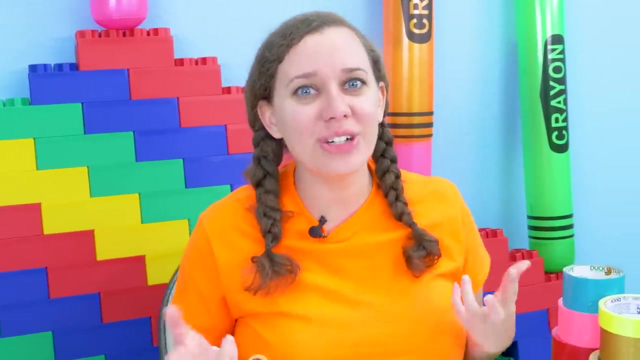 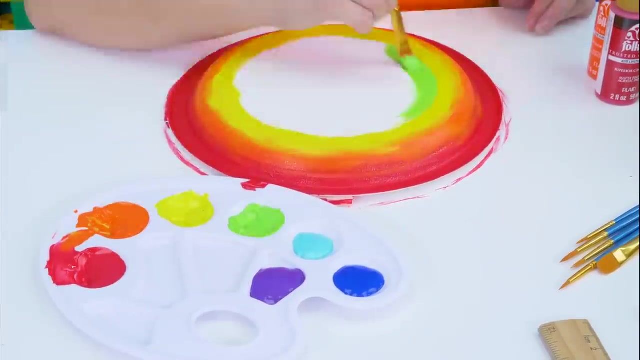 So it starts with red, and then orange, yellow, green, blue, indigo and violet, Violet. Of course, I kind of forgot your color Peck, Sorry. Whoa, Looks like a rainbow now, Cool. So the next thing we need to do is try to fold this up like a taco. 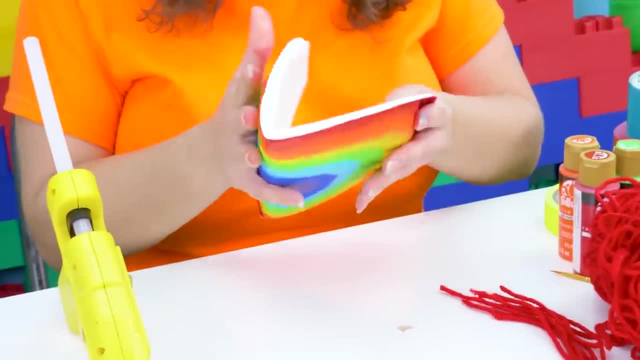 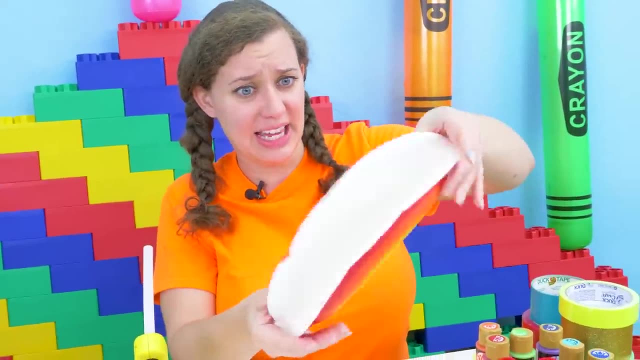 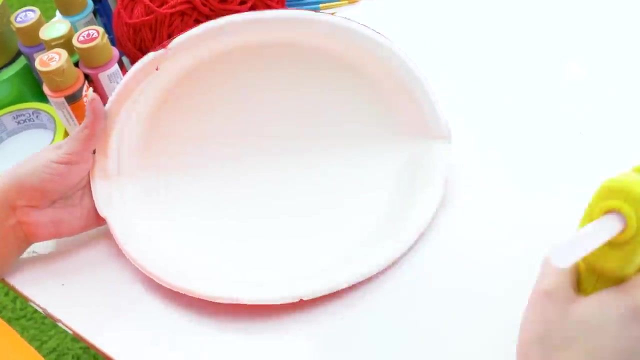 So we have only half a plate. We have a rainbow. Let's see if we can make it work. Look at that: We have a rainbow. Wow. Now I think we need to glue it together. All the glue- We need lots of glue for this, because this has got to hold tight. 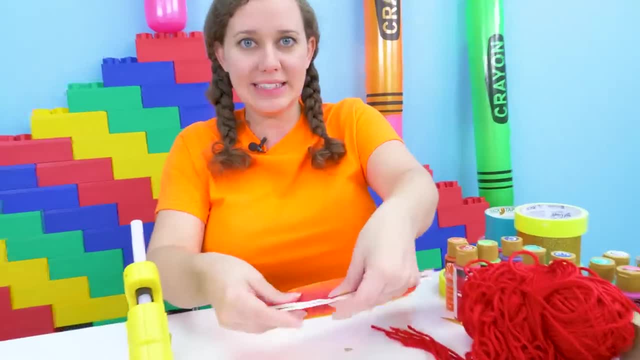 3,, 2,, 1.. And we're smashing it together. Oh, it's a little hot. This is why you need an adult for help. OK, Because hot glue can get real hot, Really hot. There we go. 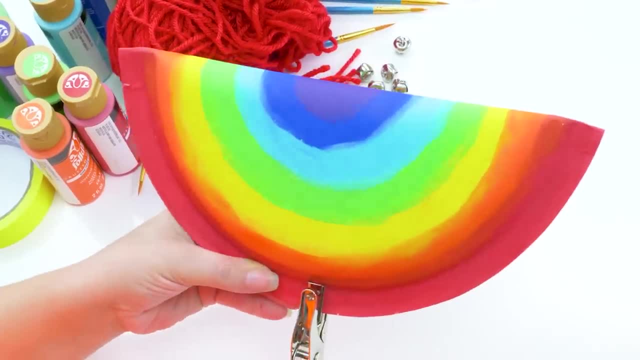 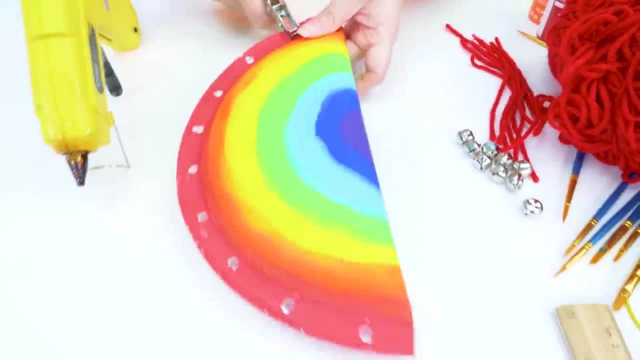 Look at that taco. Nom, nom, nom. All right, hole puncher. We need one hole for every jingle bell And last one. That was a lot of work. Now we're ready for the jingle bells. We put each bell on a string. 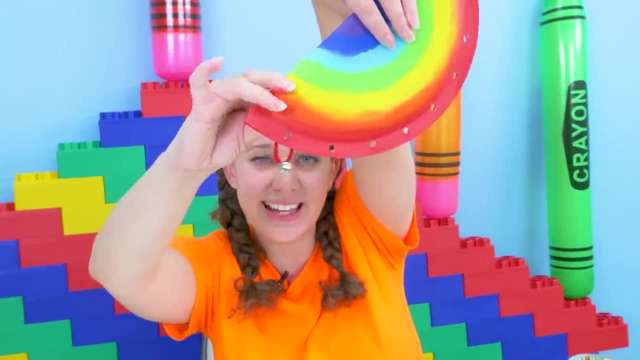 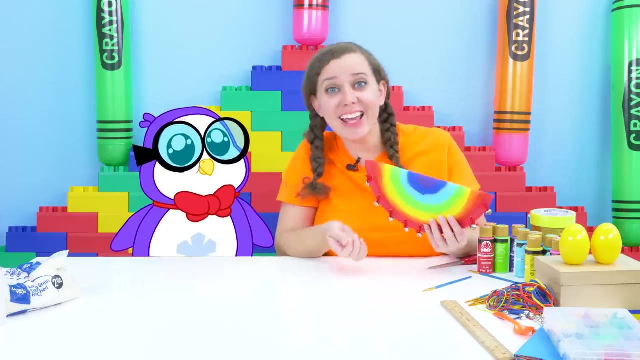 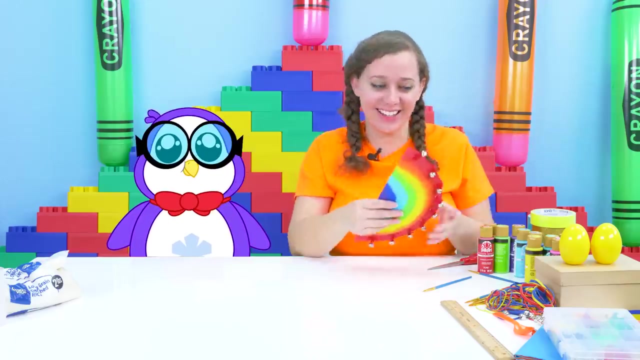 Now we're just going to take the string and tie it to each one of these little holes, like that. Ta-da And done, Ta-da, Ta-da. Now, once you have them all tied up, guess what? you have A tambourine. 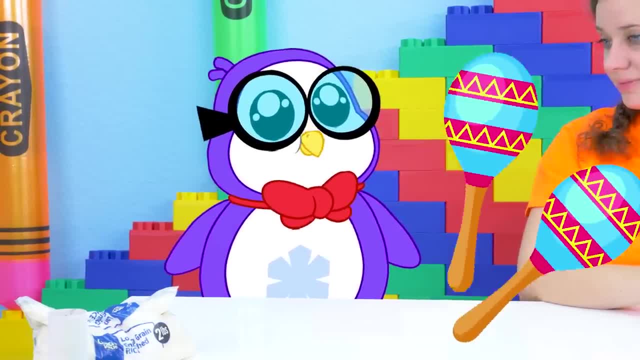 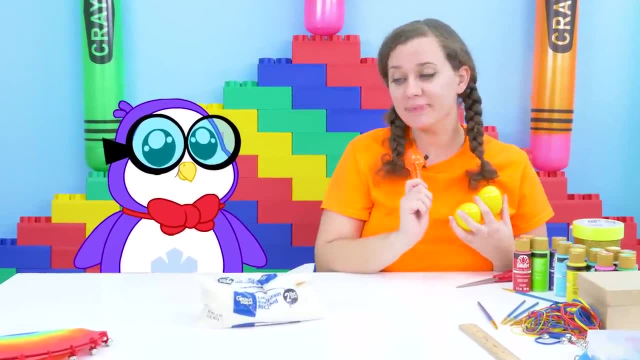 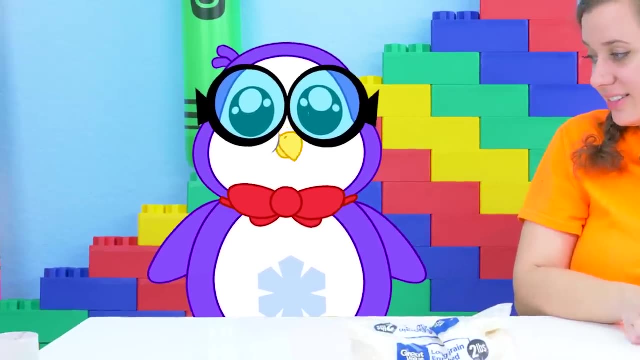 Cool, Now let's make some maracas, Yeah, OK, so for maracas, we can use these eggs that we found, some spoons, and we can use your long grain enriched rice pack, Of course, the long grain enriched rice. 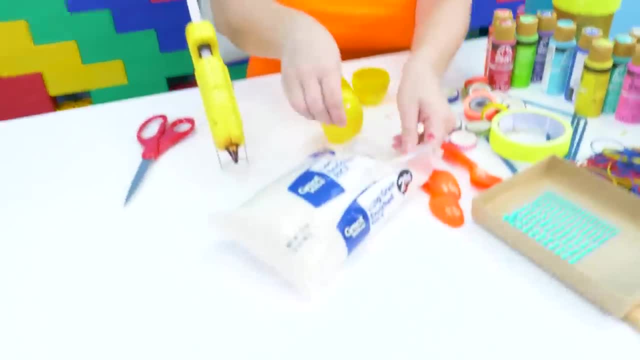 So the first thing we're going to do is we're going to put some rice in these eggs. I think I'm going to make a pickle. I think I'm going to make a mess, but it's OK. That's part of crafting. 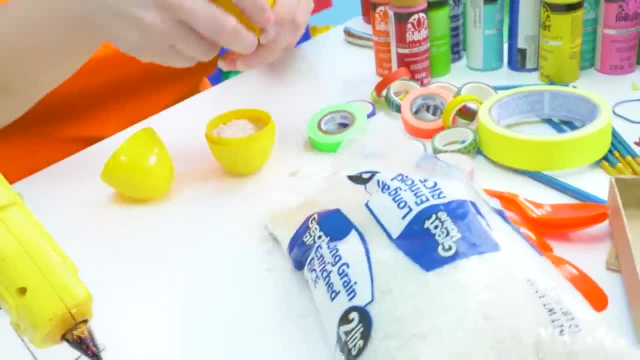 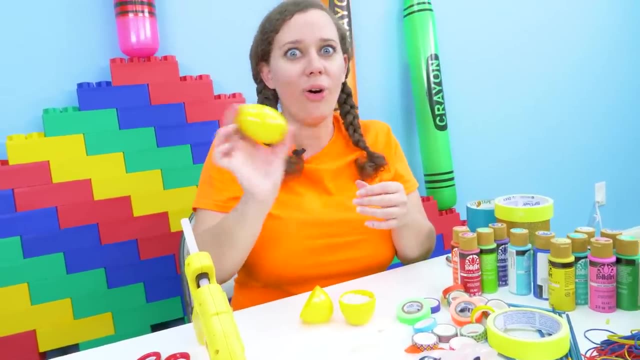 So we need some rice to make some noises. OK, I'm making a lot of mess. There we go. Now we're going to put the lids on and see if it's on. Oh, that's so cool, All right. number two now we need: 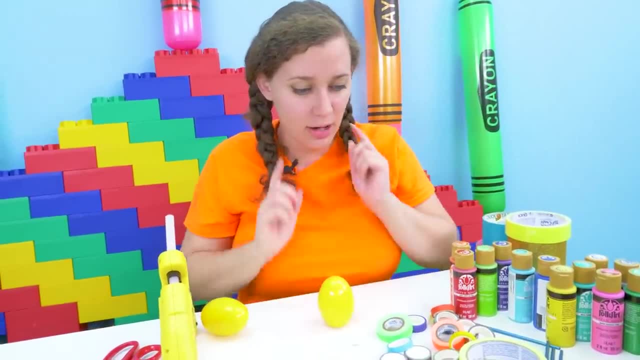 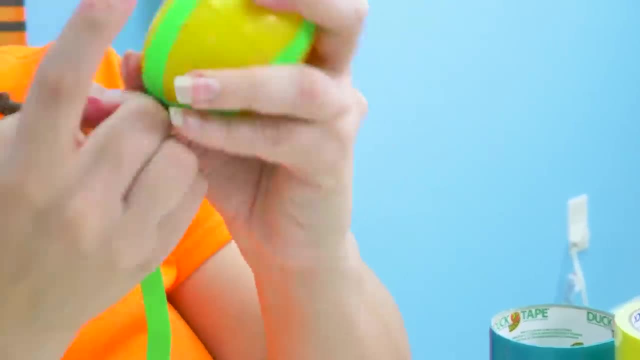 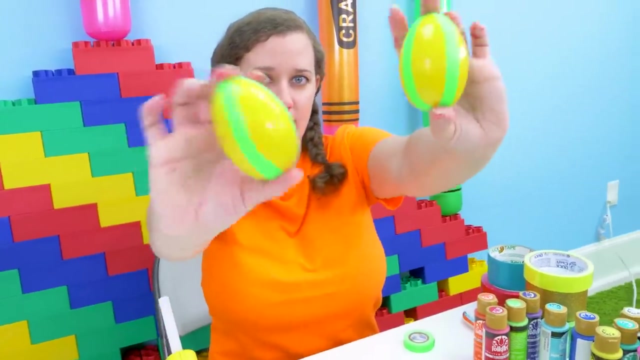 to make sure these don't open, so we don't get rice everywhere. So maybe we should use some tape, Whoa, seal it up nice and tight. That ought to be good And sturdy. Sounds good to me, All right. so now we're going to glue the spoons. 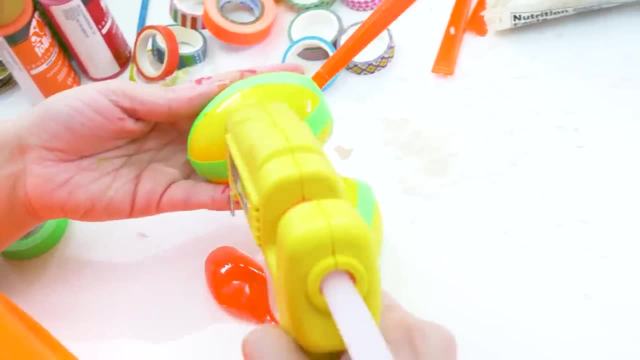 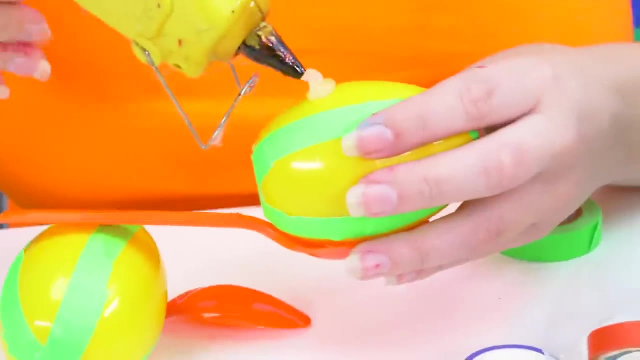 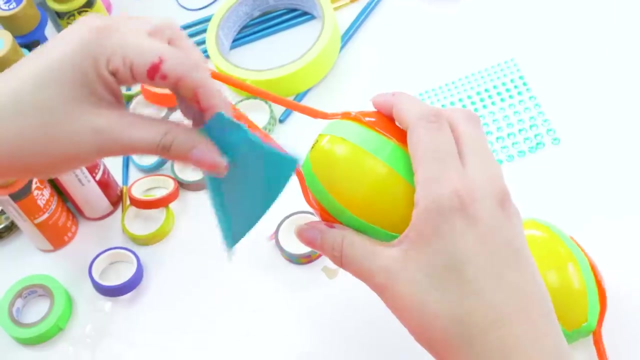 like this. to make a handle, Got to be careful with the hot glue. And oh, there we go. Handle number one, handle number two. All right, There we go. Next we're going to tape it up and then decorate. 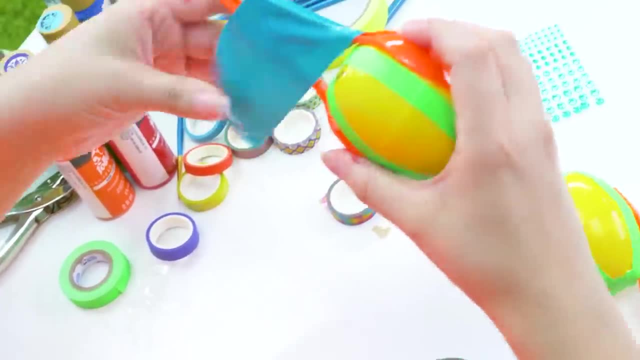 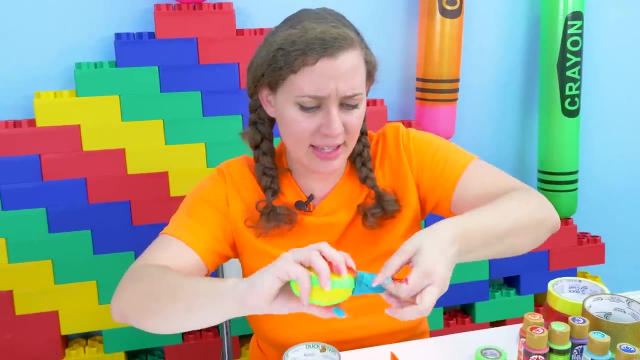 All right, taping, taping, taping, taping, taping. Ooh, perfect. Last wrap and done with that. I think we could use some decorations, though I mean they have to be festive, right Peck. 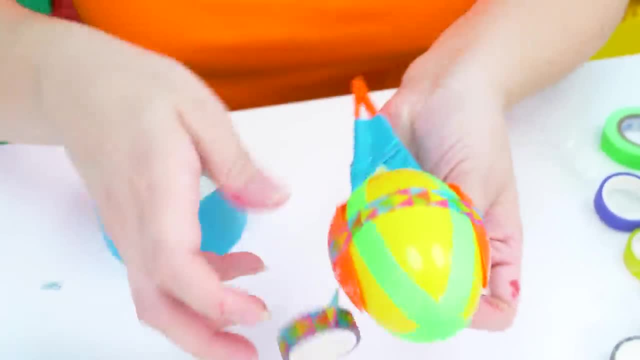 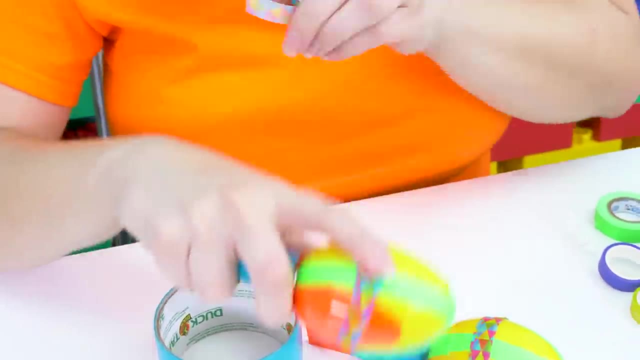 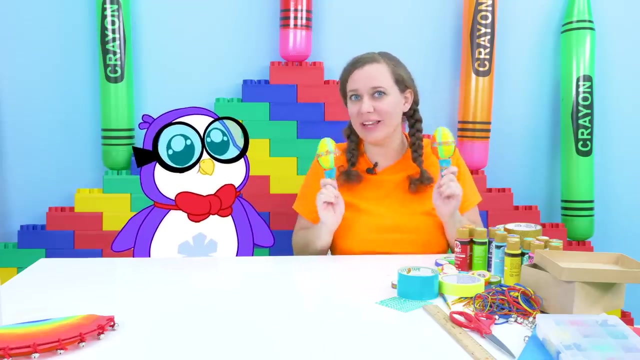 Yeah, Time for the fun tape. Oh, it's so cute. Look at all those bright colors. Super festive. There we go. Ooh, maracas, spectacular. Yes, I mean, the festive tape is definitely what made the maracas, so listen to that. 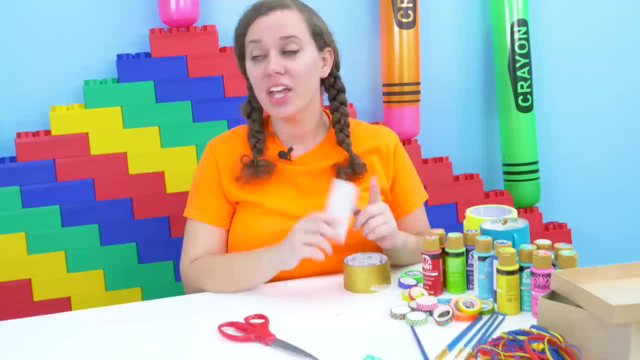 OK, well, next we can use the toilet paper roll for something You know what Peck. I actually have an idea for the toilet paper roll, but it's going to be a surprise, So you're just going to have to wait and see what it is. 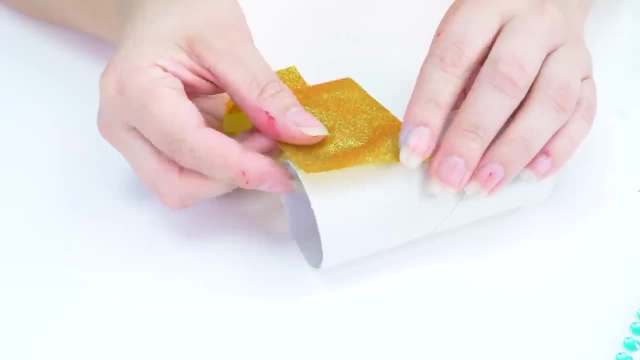 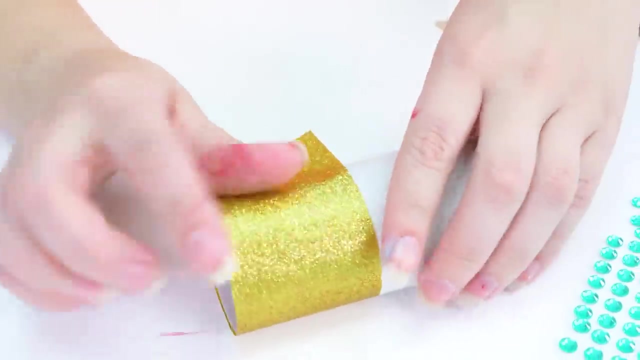 We're going to start with this super shiny, sparkly tape. OK, so just because we don't want it to look like something that came from the bathroom, we're going to wrap it in this super shiny tape. Ooh, that's so pretty. 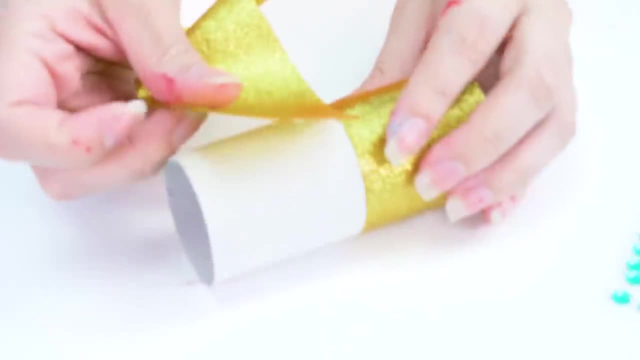 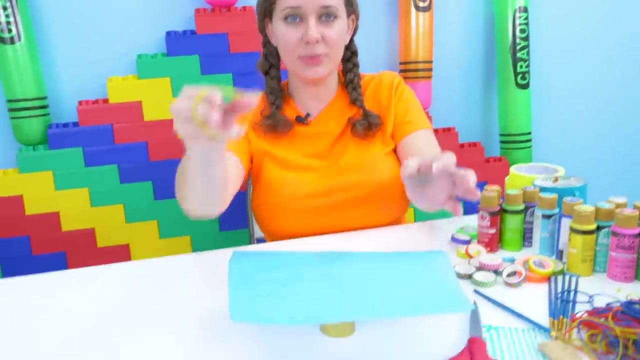 All right, Let's cover this other end. There we go. We're going to take the tissue paper, crinkle, crinkle, crinkle, and put it on the edge of this with a rubber band. Ready Dun dun. 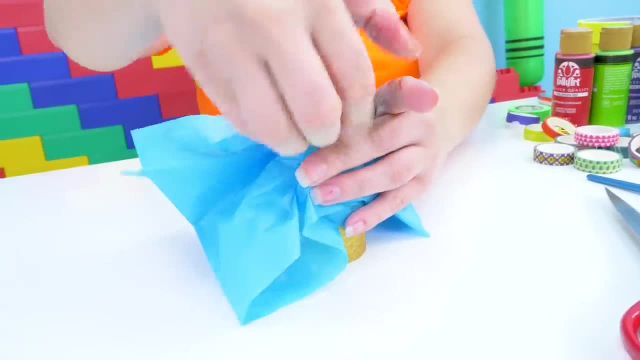 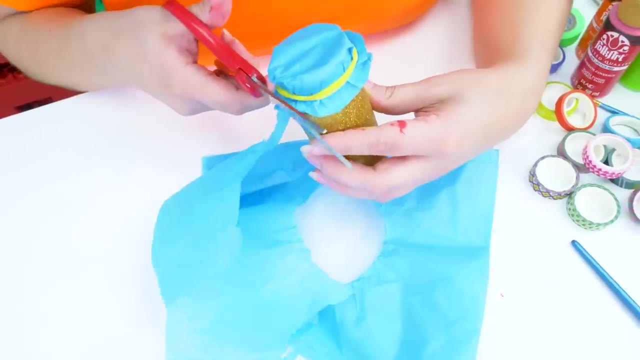 The science of rubber, banding things together. super technical. There you go. Well, now we can't really see our kazoo, so maybe we should trim this up some. Oh, that looks so much better. Now we can actually see our kazoo. 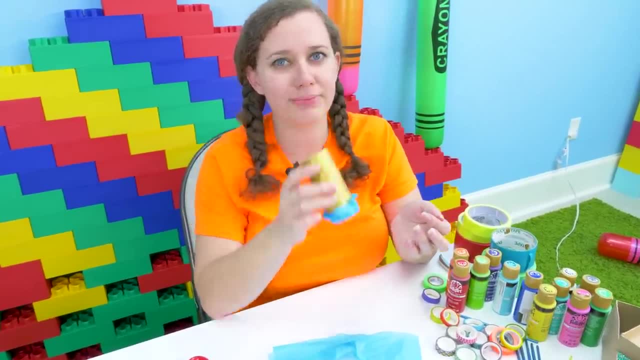 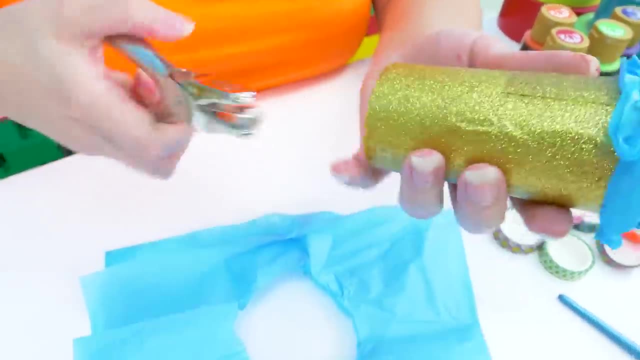 Da, da, da da. Oh da, We're catching a little bit of air here, so I think I have the perfect thing to help us out. We just need to make a little air hole. Oops, backwards Bink. 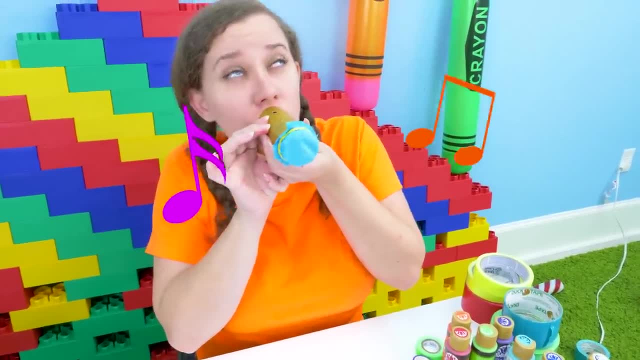 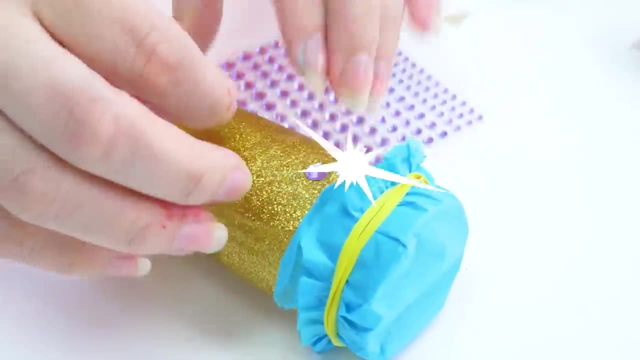 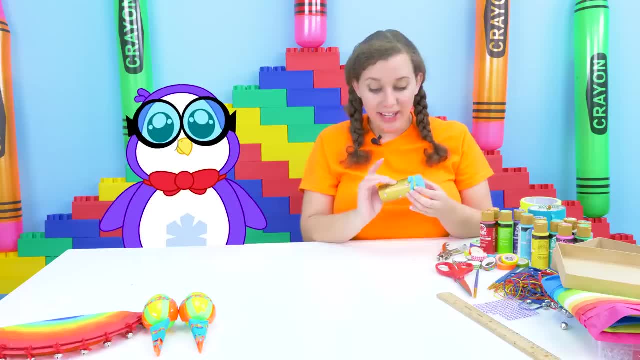 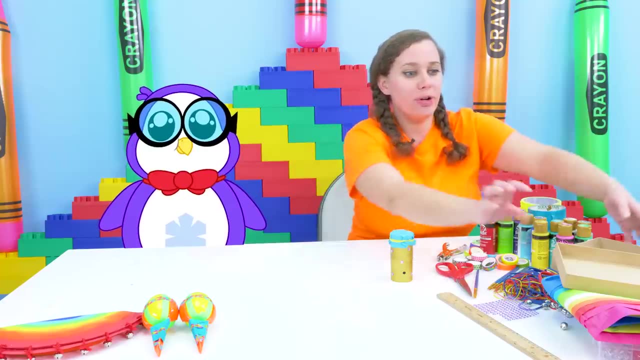 why not just decorate it a little bit, you know, for some extra credit? We got all our jewels on Peck. what's next? The last one will be tricky. A guitar- Ooh, I have the perfect body for that guitar. 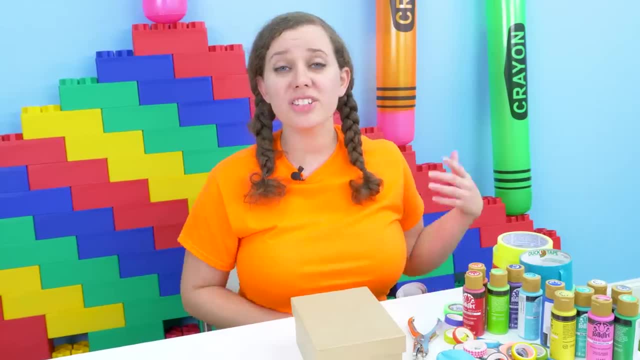 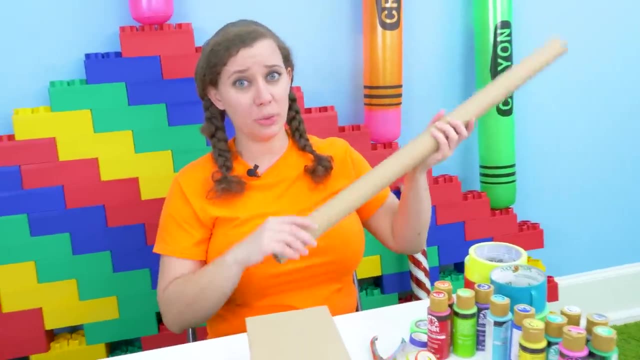 What about this? That'll work, So we're going to start with the neck of the guitar, which we can actually use: the wrapping paper roll that we found. This is a little long, so we're definitely going to have to shorten it. 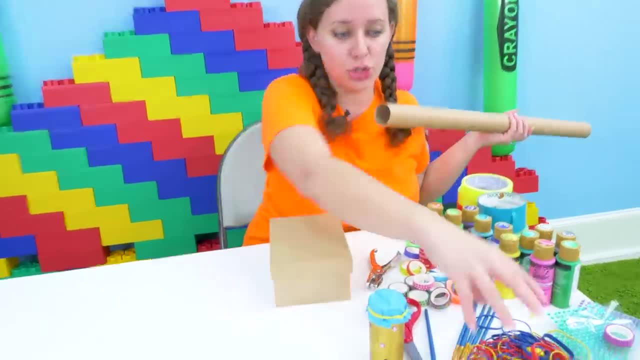 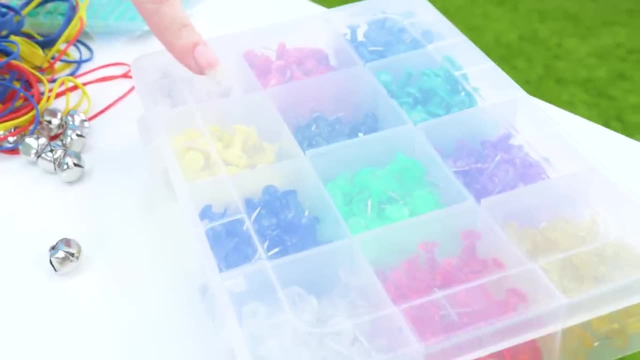 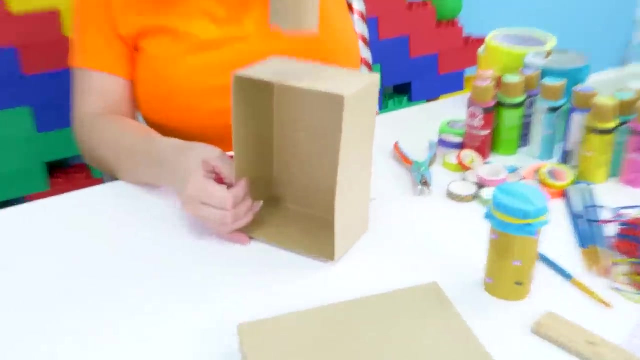 And then we have our body, which is this box. We have strings to pluck and play with, and I think we even have little tuning knobs that we can use. Yeah, Hi-yah, Perfect length. What a coincidence. So now we just need to cut a hole so we can stick this guy through it. 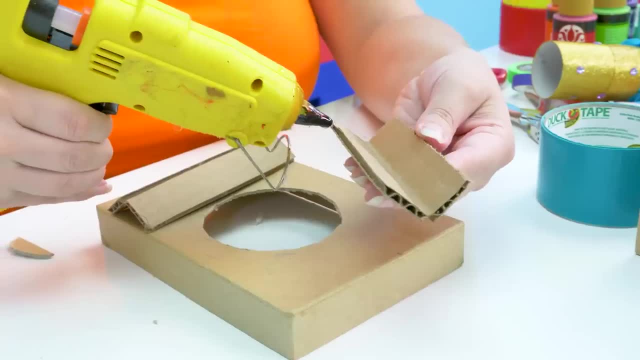 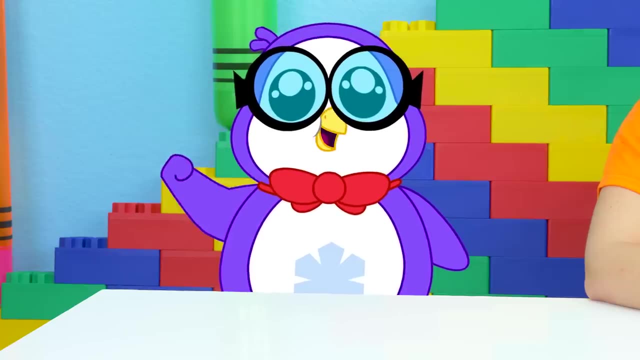 Bing Perfect hole. So we're going to use these pieces of cardboard as string holders to hold our strings in place, All right, While we're waiting for the glue to dry right here, which this is what's going to hold our strings in place. 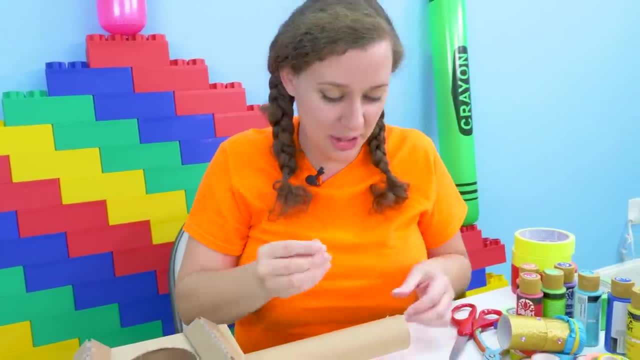 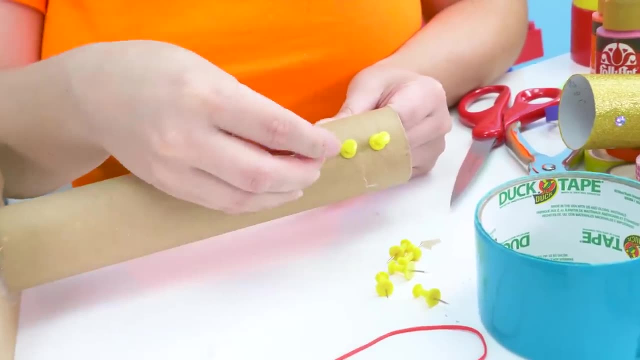 let's put some little tuning knobs. Of course they're not going to work, but I think it'll really help it look like a guitar. So we need six of them: total One, two, three, Awesome. And then the other side. 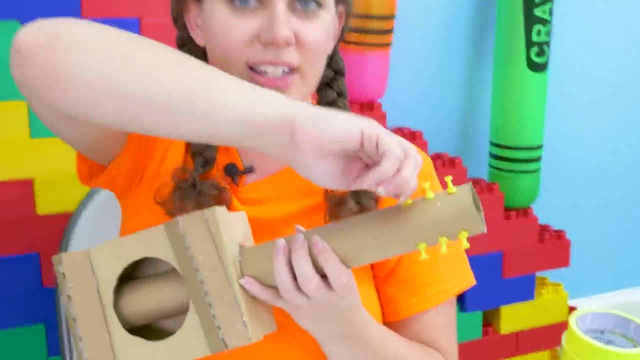 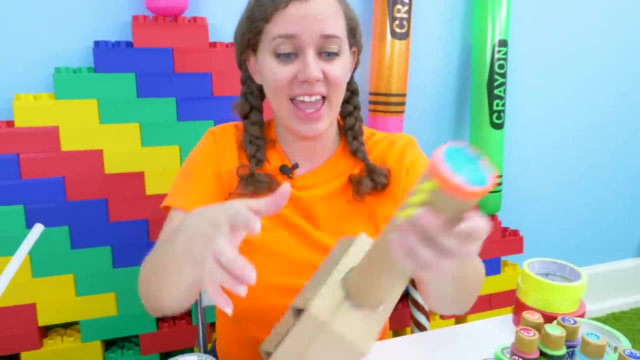 There we go That way. when it goes out of tune, you can just tune it up Just like that. So we sealed up the ends. That way you can't get poked by any of the thumbtacks. And now I think we're just ready for the strings. 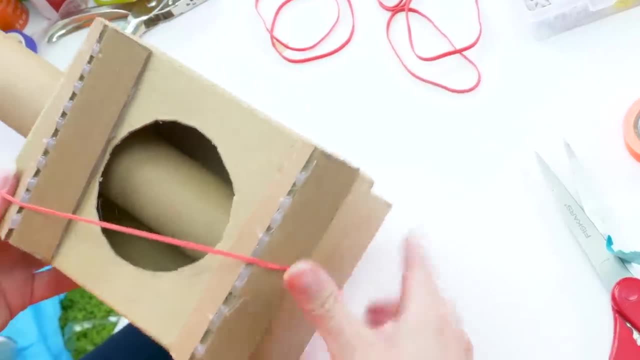 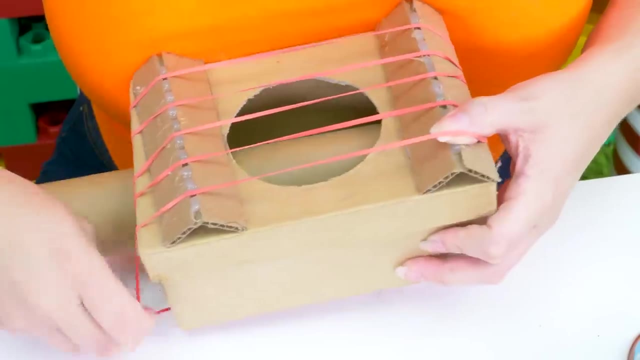 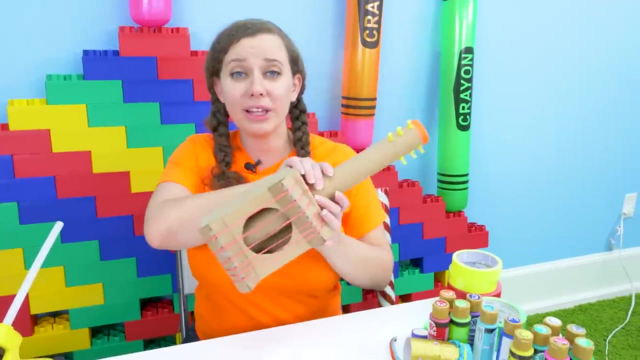 All we have to do is put the strings on the guitar very carefully, Make sure we don't pop any. There's five And our final string, string number six. You want to see how it plays. You recognize that song, right. 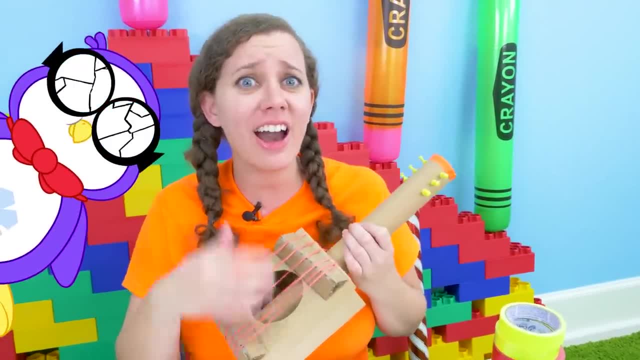 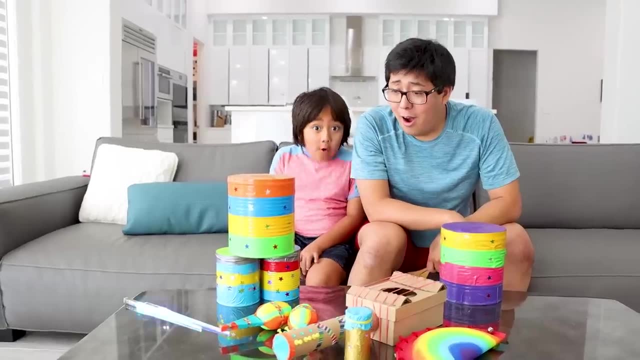 Twinkle, twinkle little star. How, I wonder, Whoa? Thank you so much, Peck. Those are so cool. I'm going to test them out. I'm going to test out this guitar. Whoa Cool. 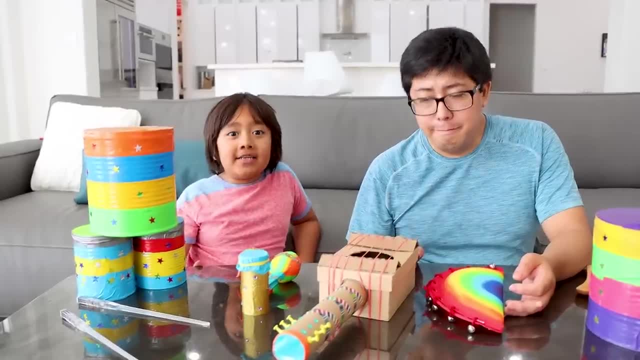 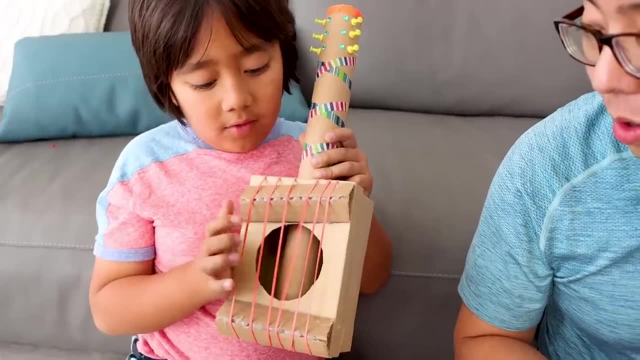 Does it make a sound? Yeah, They all make different sounds. Whoa, Look, Ryan, This tambourine also make a noise. Whoa, Let's see, Let's see. Whoa, Whoa, Whoa, Whoa. 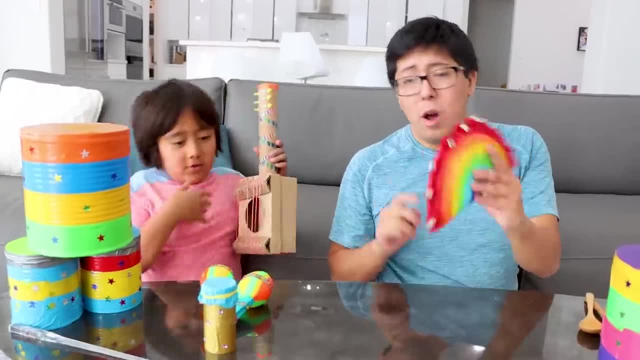 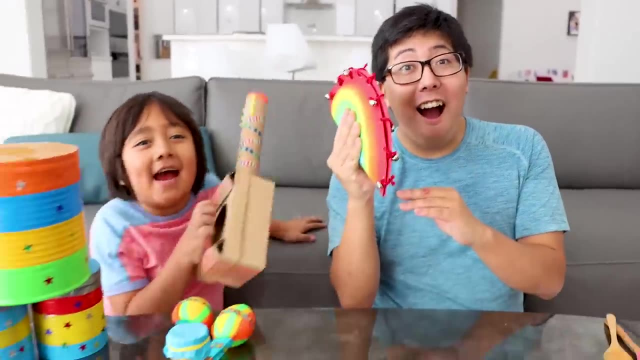 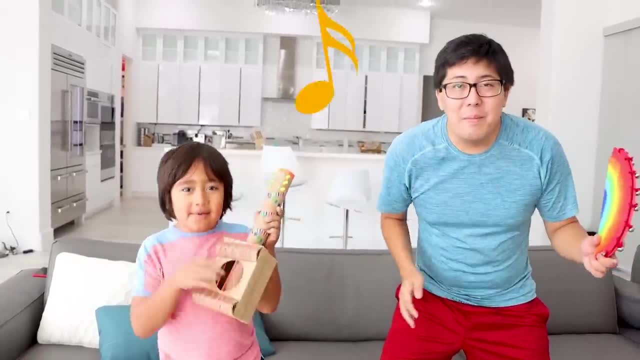 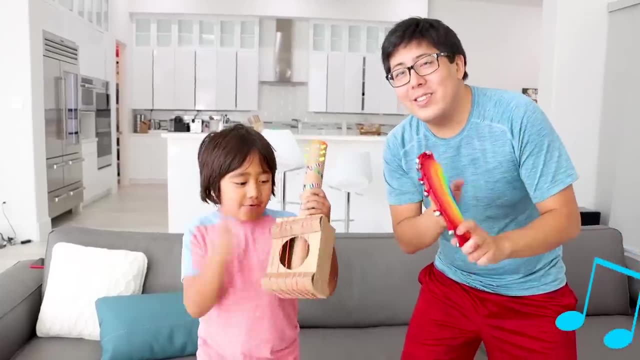 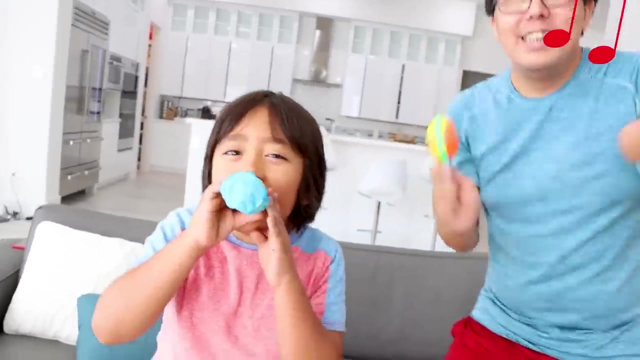 Lets jam. Happy Birthday to you. Happy Birthday to you. Happy Birthday, dear Zombie, Somebody out there. Happy Birthday to you. Woo, Wow, Wow, Wow. I have two hands. Two, two, two. I have two hands. 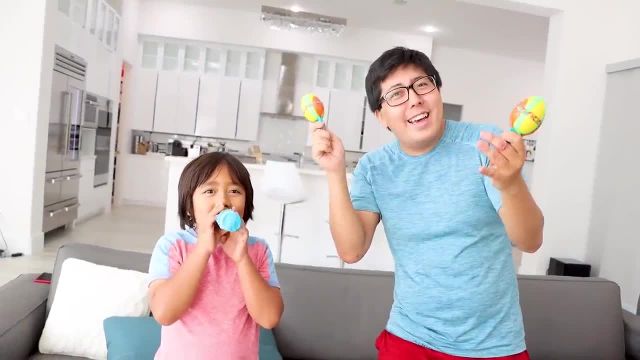 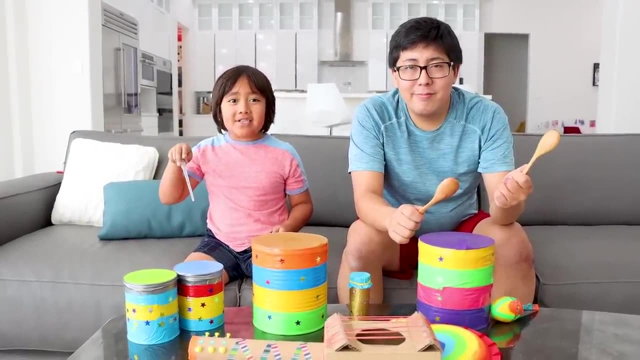 Two, two, two. I have two hands. Two, two, two. I have two hands. I forgot the rest, our do-it-yourself instrument video, And if you're at home maybe you can try to make these too.